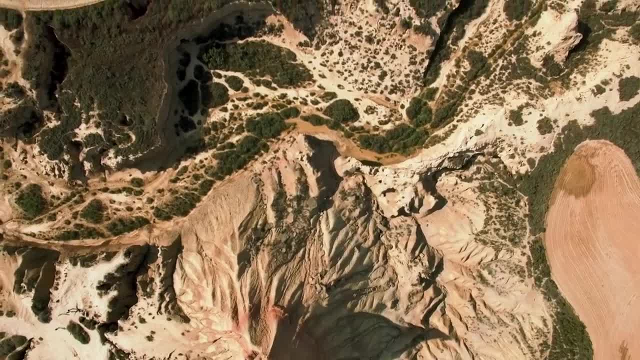 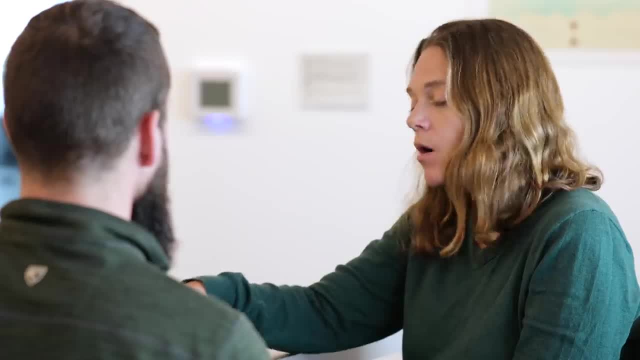 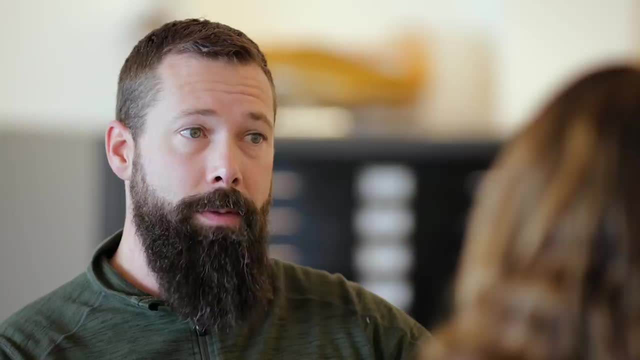 it through tunnels that are miles long, through the mountains, into reservoirs and then either into rivers or pipelines. That's something that a lot of our students have never actually thought about before. So how are you managing water? here? We've reduced water usage by 38 percent, which is a pretty big drop. I think it's the 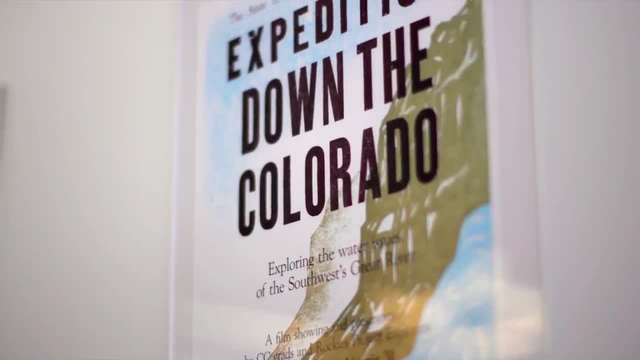 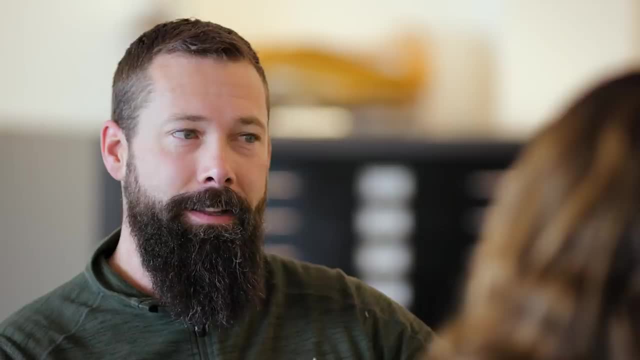 biggest in the country, actually Multiple different ways: The fixtures, low-flow showerheads in our residence halls and low-flow toilets, things that aren't shiny, flashy, exciting things, But as we add all of those together, they start to have a really big impact. 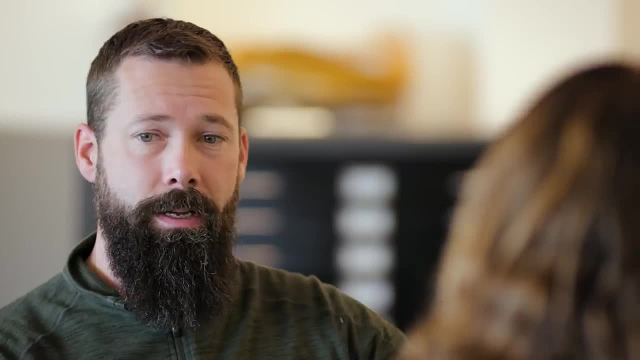 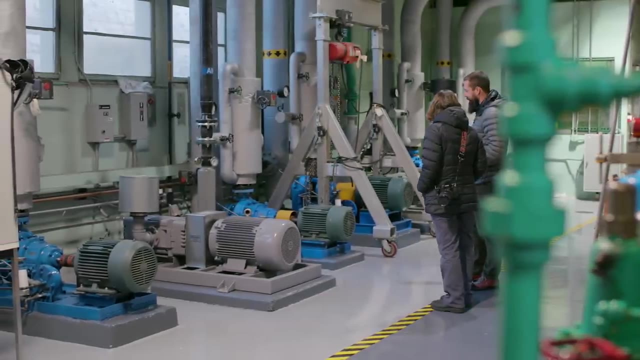 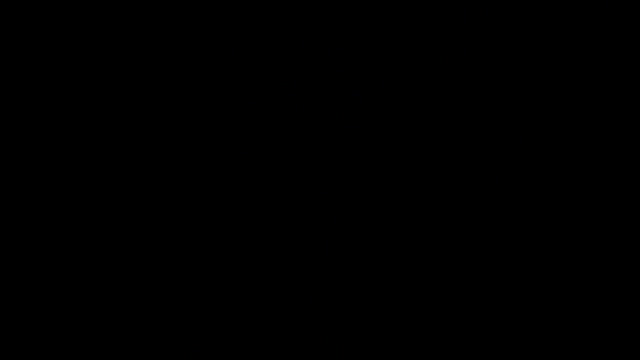 And then just efficiencies. There's a lot of technical projects that we've done. One of the projects that has saved a lot of water Okay Is the cooling system for our central heating plant. We closed the loop on that. That saved us about three million gallons of water a year. 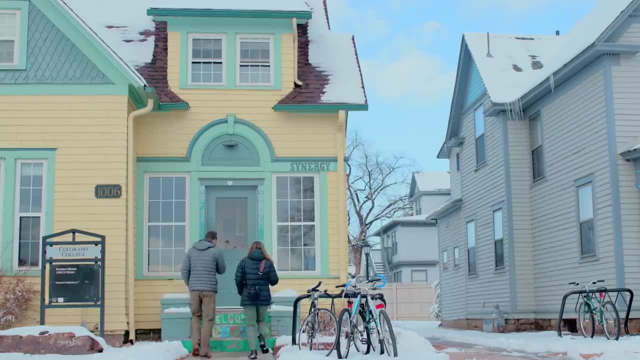 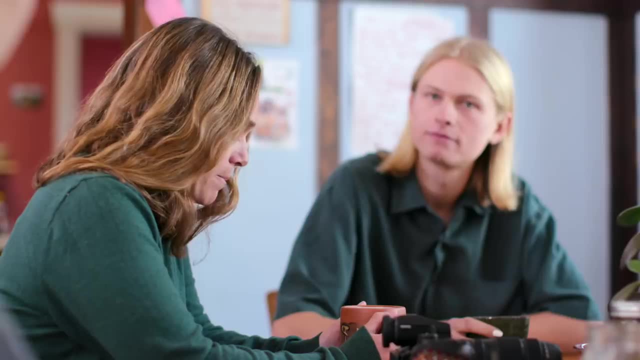 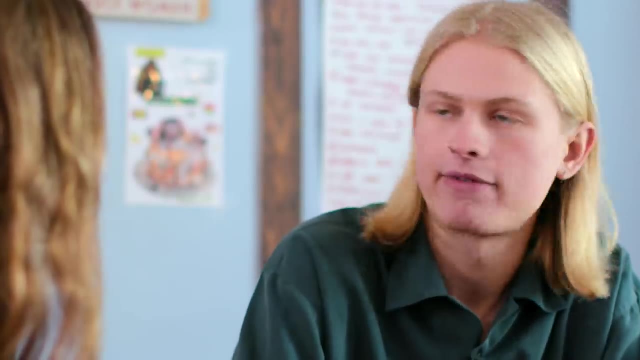 There are many lessons we can learn from Colorado College. I'm here in the college's eco-home with a family of students who are learning more about being water-wise. Talk to me a little bit about Synergy, your relationship to water. Here at Synergy, we do use gray water. When we shower we have like a five-gallon bucket. 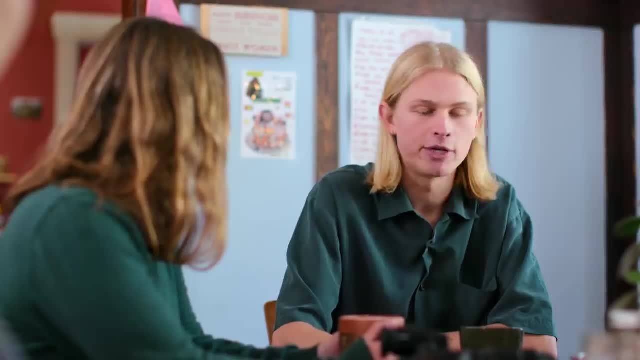 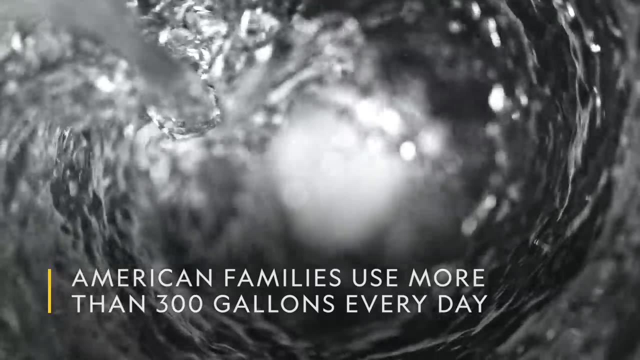 We have a bucket below us that we kind of just let fill up while we're showering, And then we use that to like flush the toilet. So about half of our indoor water use is spent in bathrooms, with showers as the major drain. On average, American families use more than 300 gallons of water every day. 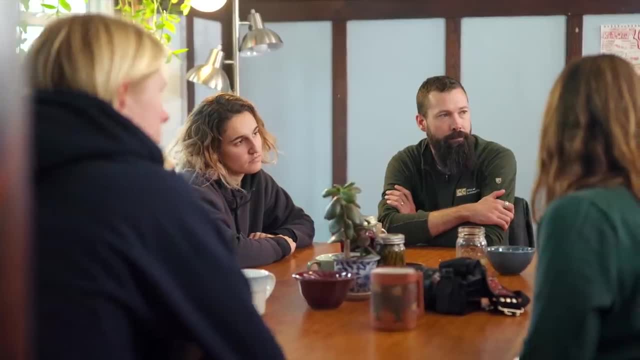 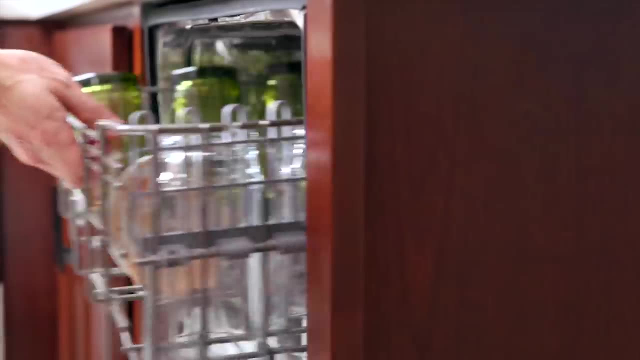 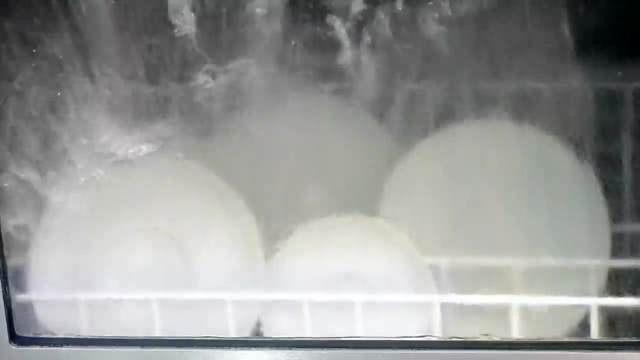 Wow. And many of us still rinse our dirty dishes under a running faucet before loading them into the dishwasher. This is a huge waste of water, because you actually need the dishes to be dirty, as the enzymes and the detergent latch onto food particles to work effectively. 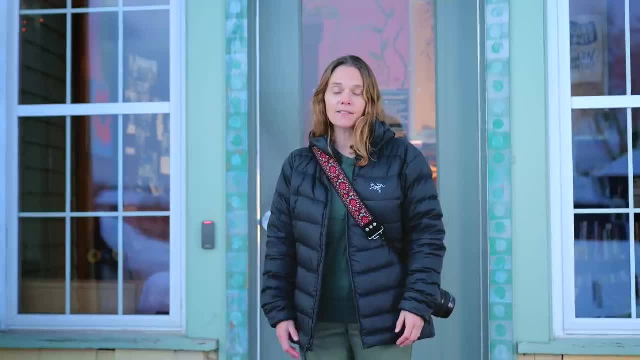 And it's these actions that could help avert America's looming water crisis, giving the next generation a better chance of never having to see a water shortage.